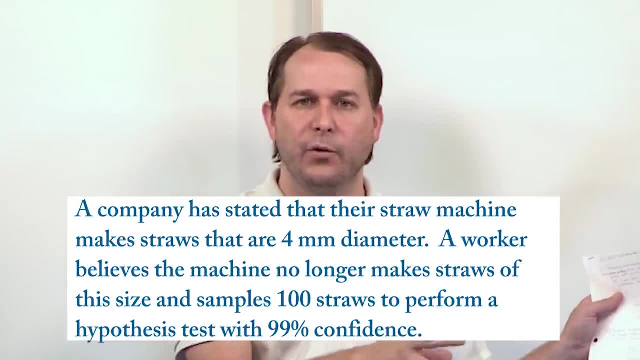 millimeters or anything like that. It just says that the company believes the straws are four millimeters or anything like that. It just says: originally everybody thinks it's four millimeters, The new guy thinks it's not four millimeters. So that's important because some of 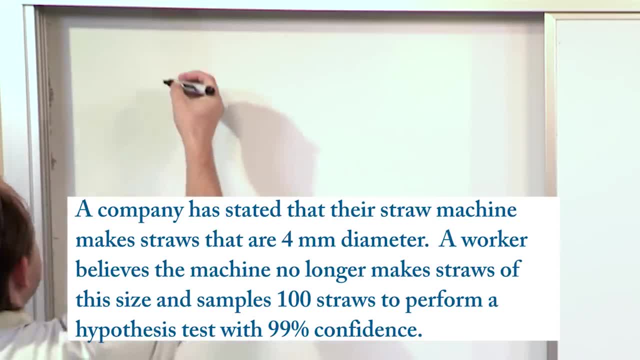 these problems are going to have greater than or less than Some of them won't. So in this case, the null hypothesis is what kind of the status quo belief is, And you can see from the very first sentence what we're talking about is the mean, okay, the average value for the diameter of these. 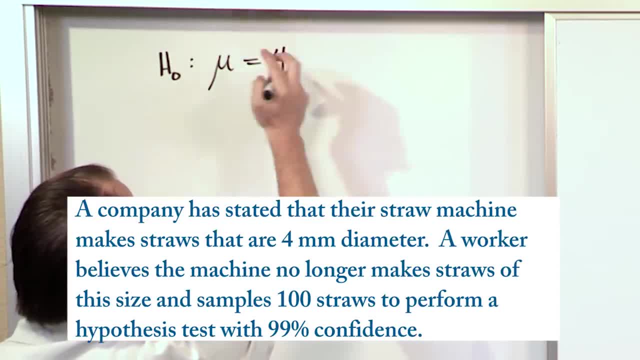 soda straws. And the default hypothesis or the null hypothesis is that everyone thinks the straws are four millimeters. Okay, but then when you read the next sentence, an employee believes that this is no longer the case. So the alternate or the research hypothesis: the new guy thinks that it's no longer. 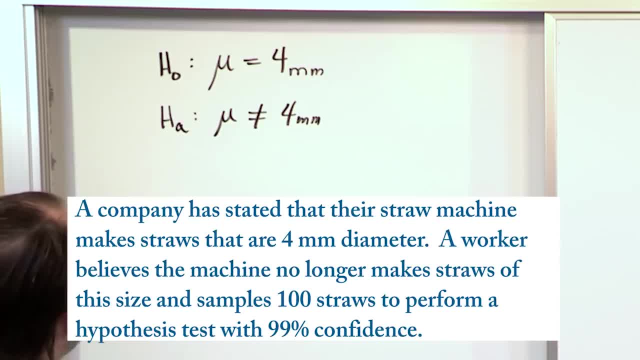 four millimeters. So on a test or a quiz, when you're asked to write down the null hypothesis and the alternate hypothesis, this is what you're asked to do. The null hypothesis is sort of the default belief- innocent until proven guilty, so to speak- that the soda straw machine makes straws. 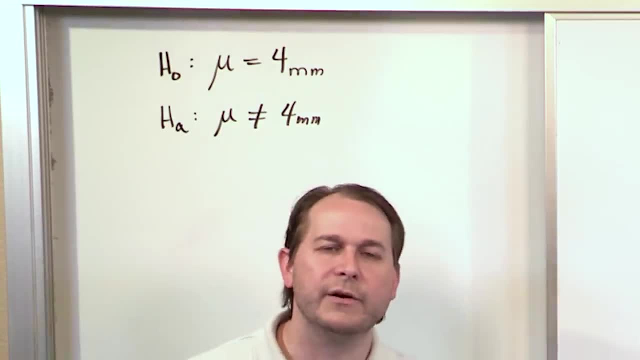 of this diameter. The new guy comes along to challenge it and says no, no, no, it actually isn't producing straws of that size, And we have something like this. Notice that these guys are mathematical opposites. Every possible scenario is contained when you look at the total of the null. 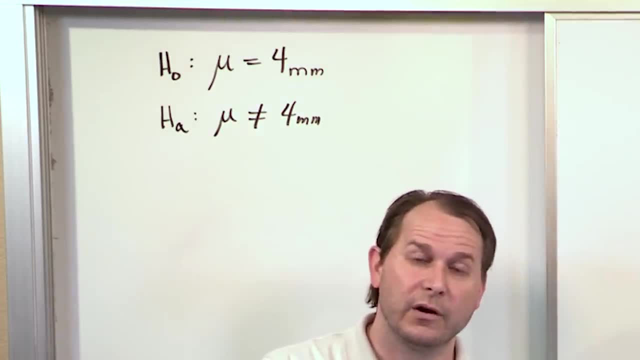 plus the alternate hypothesis, In other words, either it's four or it's not four. That would encompass any size straw, So they have to be mathematical opposites And when you take them both together it's going to cover basically all possibilities of what the machine might be doing. 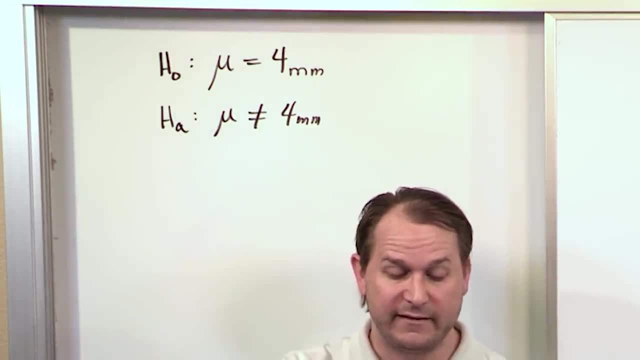 Notice we don't have any greater than or less than here, because the actual problem doesn't say anything about greater than four or less than four. It just says four millimeters or not four millimeters. So you need to read everything carefully. All right, So this is really the. 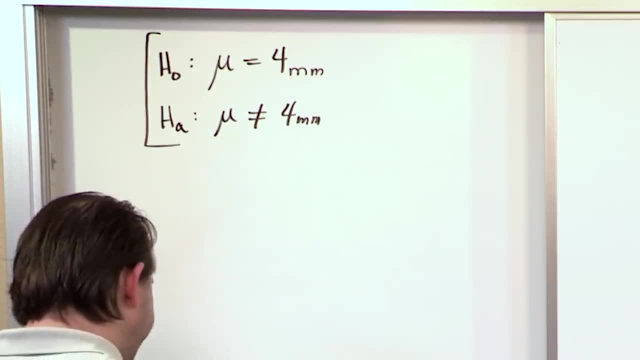 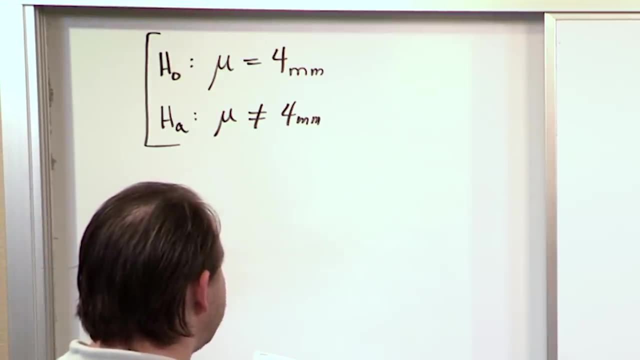 answer to the problem All right, But I want to go just a touch further and just kind of discuss. if we read a little bit more into the problem, it says we're going to test this by taking samples of 100 straws. So as we go further in the hypothesis testing, you'll need to know how. 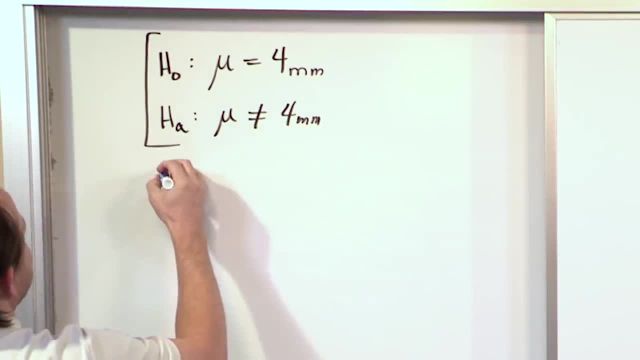 many samples did you actually choose to test the hypothesis? And that's usually the variable n. In this case it's 100 samples. And it also told us that we wanted a 99% confidence. So that means that the variable c is 0.99.. When you have 99%, you need to put it as a decimal. That's what the 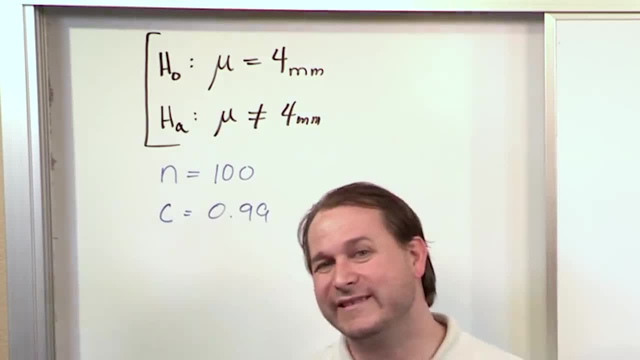 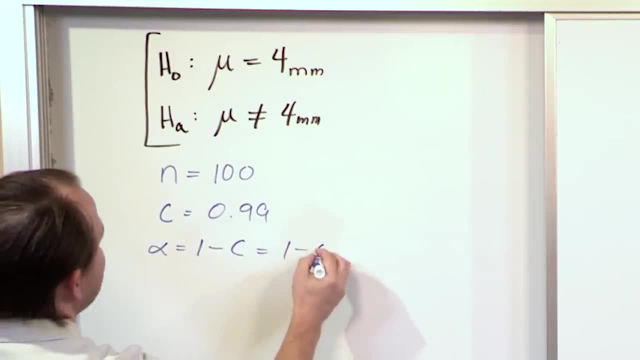 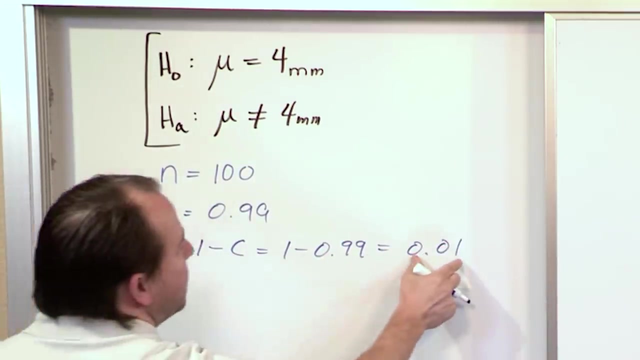 value of c is OK. Now I told you, sometimes we're going to be using c, Sometimes we're going to be using alpha. All right, Alpha is just simply 1 minus c Minus 0.99. So 0.01.. So if c is 0.99, alpha has to be 0.01.. So when c is very high, alpha is very. 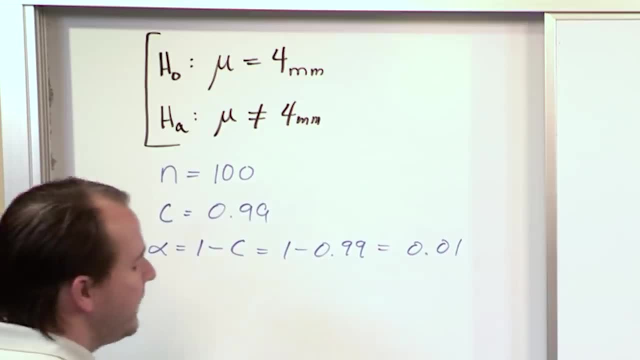 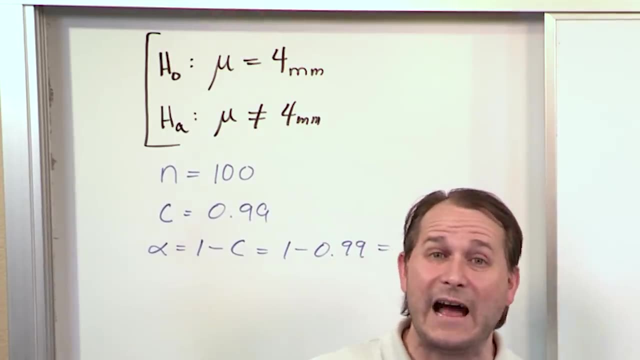 low. When you add these guys together, you're always going to get 1.. So it doesn't really matter if the problem tells you the level of confidence c is 99%, or if it tells you the level of significance alpha is 0.01.. It's telling you the same exact information. Alpha and c are directly. 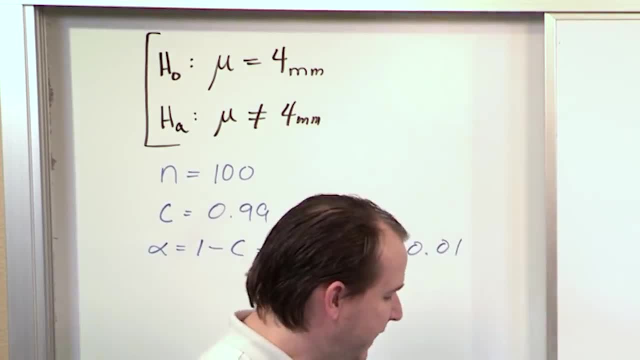 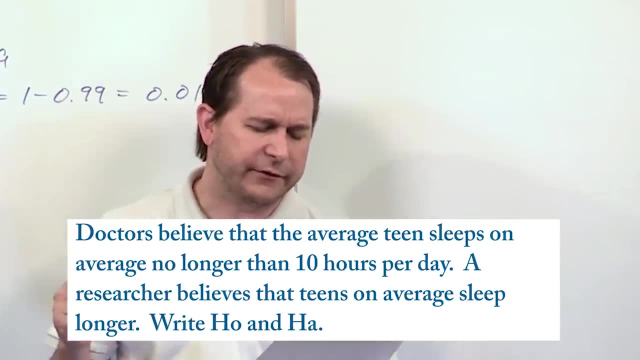 related, because they have to add up to be 1.. All right, So again, we're not doing the test thing in this problem or in these problems, We're just writing the hypothesis down. The next one: Doctors believe that the average teen sleeps, on average, no longer than 10 hours. 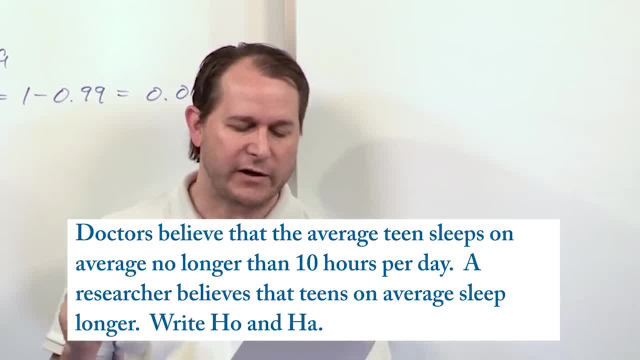 per day. A researcher believes that the teens, on average, sleep longer than this. We want to write down the null and the alternate hypothesis. Now the difference in this case is: notice, the wording is very different. Doctors believe that the average teen sleeps no longer, no longer. 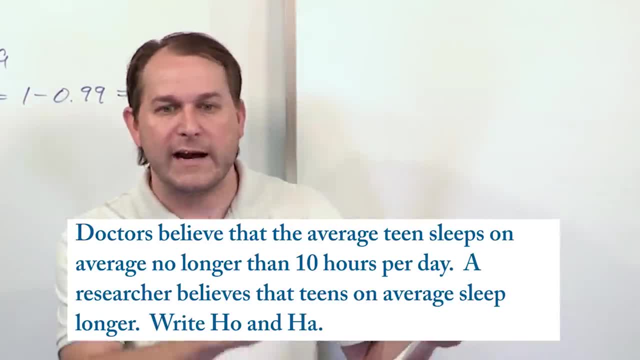 no longer. That means that doctors believe that they might sleep one hour, two hours, three hours, four hours, five hours, But as soon as you get to 10 hours, no longer than 10 hours means no longer than that. So this is clearly not a case when we have equals. 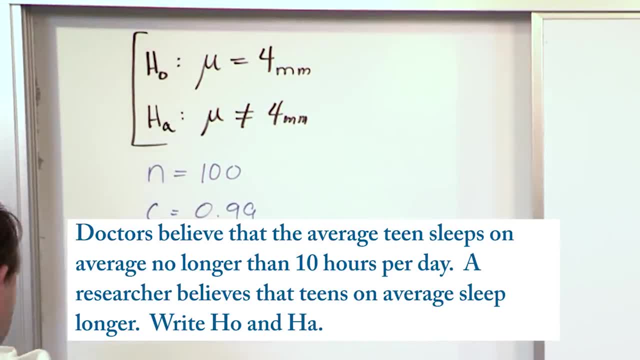 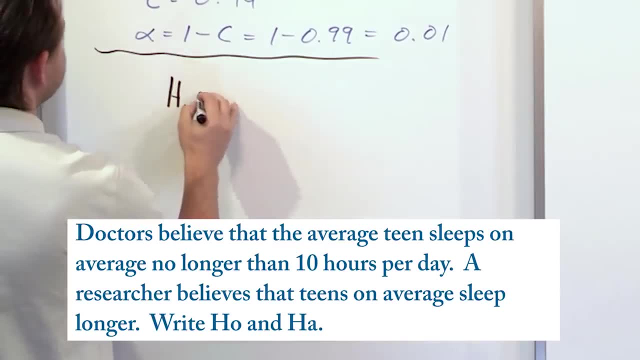 or not equals, because the wording of the problem is telling us no longer than 10 hours, So we're going to write the null hypothesis accordingly: Null hypothesis. We're going to use this symbol, mu, again, because we're talking about the average amount of time that 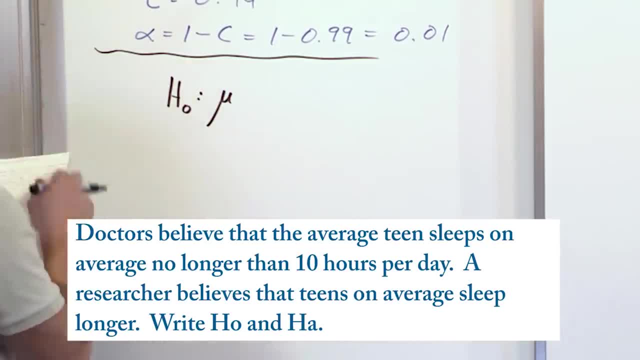 teens sleep. So this is what? Well, l is equal to the time, on average, that entire section of the brain's, on average, that each of the homemates sleep. So this is what you notice. excuse me, These are. So this is a mean, this is a mean value. for the population of teens Should be less than or equal to 10 hours. Make sure you understand this. The first sentence. doctors believe the average teen sleeps, on average, no longer than 10 hours. Less than or equal to. that's what this means. 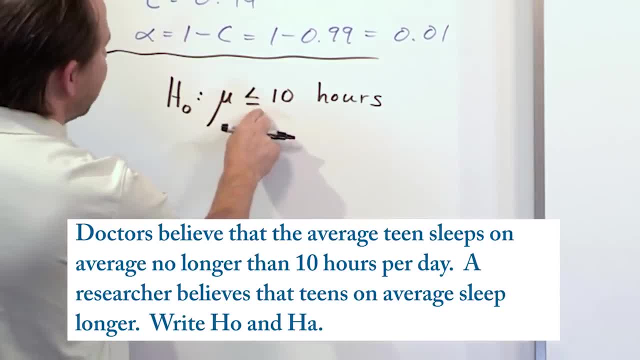 So one, two, three, four, five, six, seven, eight, nine or 10 hours because of the equal sign here. 10 hours, but no more than that, And that's what this is saying. The mean is less than or equal to 10 hours. 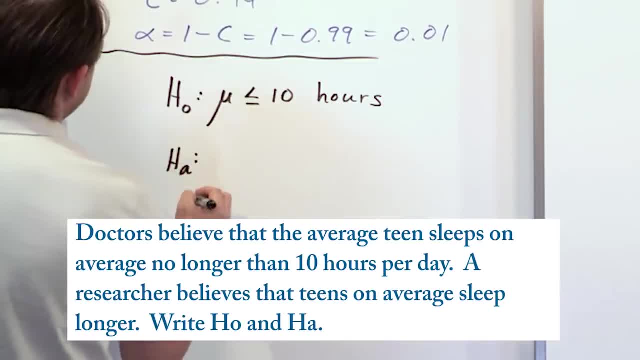 So if this is the case, what would be the alternate hypothesis, or the research hypothesis, or the challenge hypothesis? Well, if it actually says a researcher, who's the challenger, believes that the teens on average sleep longer than this, that means that it has to be greater than 10 hours. 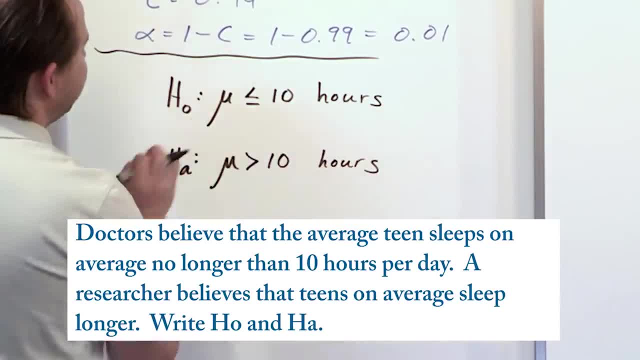 So if you were asked on the test, write the null on the alternate hypothesis. this is what you would be expected to write. The null hypothesis is saying that the teens do not sleep any longer than 10 hours, So any amount of time up to 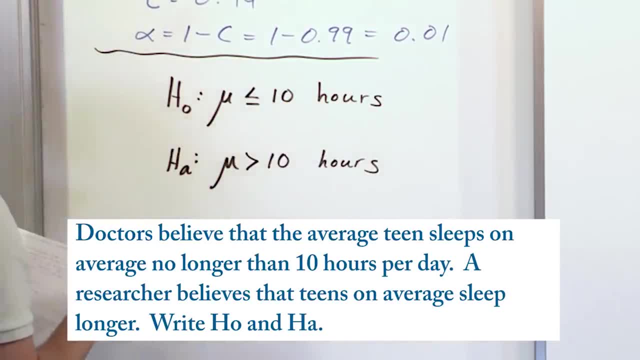 and including the average teen, including 10 hours. that is what we call the null hypothesis. But the researcher comes along and says no, on average, I think teens do actually sleep more than that, So we have to have a greater Notice. there's no equal sign here. 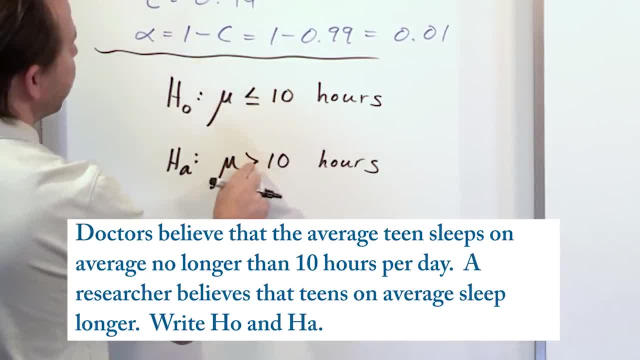 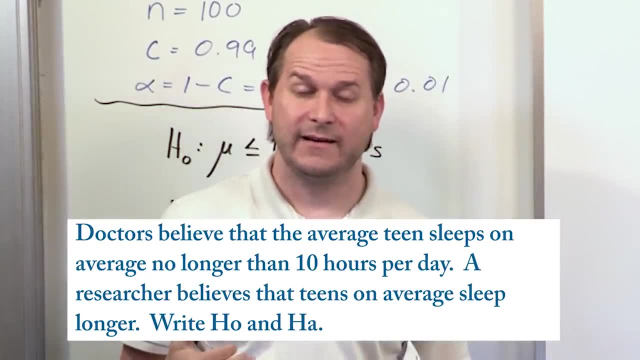 because the equal sign was here. So, all the way up to and including 10 hours, this would be 10.1, 10.2,, 10.3 hours, 11 hours, 12 hours, anything greater than 10, right. 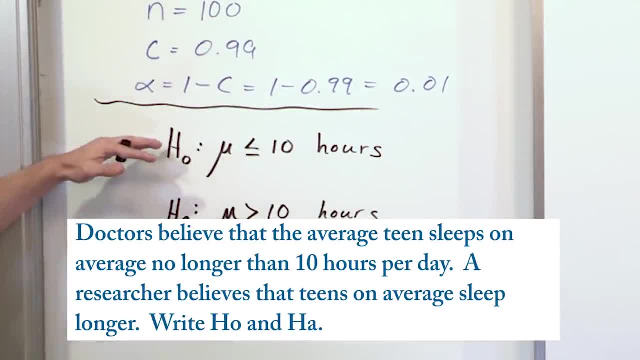 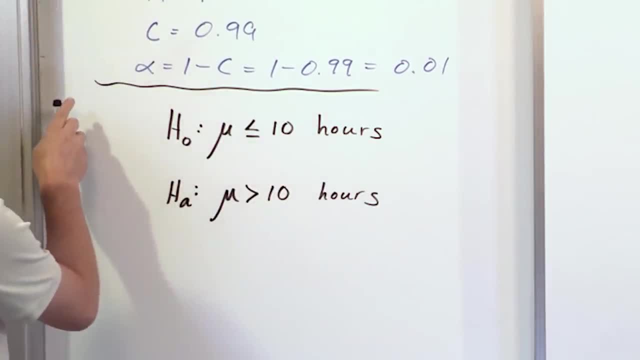 And then exactly 10 would be included here. Also notice that the null and the alternate hypothesis are mathematical opposites of 10.. In other words, the first hypothesis includes every number up to and including 10.. The second one includes all numbers beyond 10.. 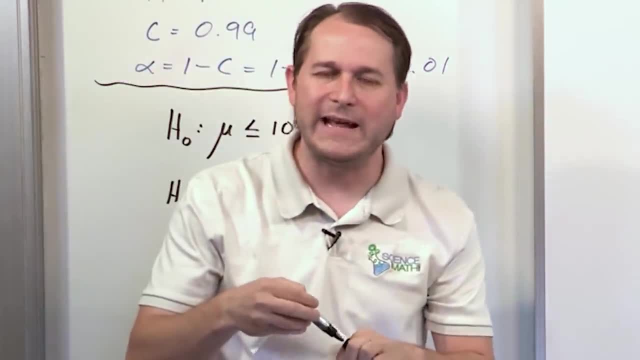 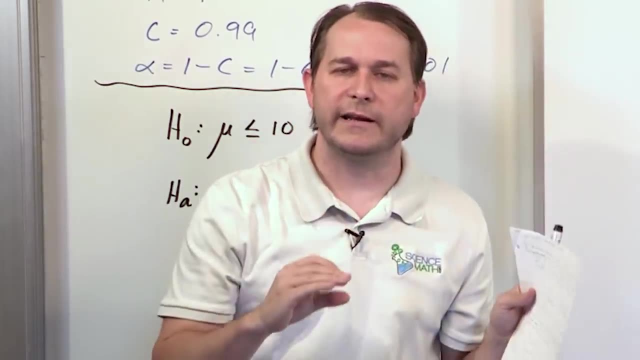 So together they include basically all possible answers for how many hours a teen could possibly sleep, And that's how all of these hypothesis tests are going to be set up. When you construct the null and the alternate and you look at it together, it should encompass all possible answers. 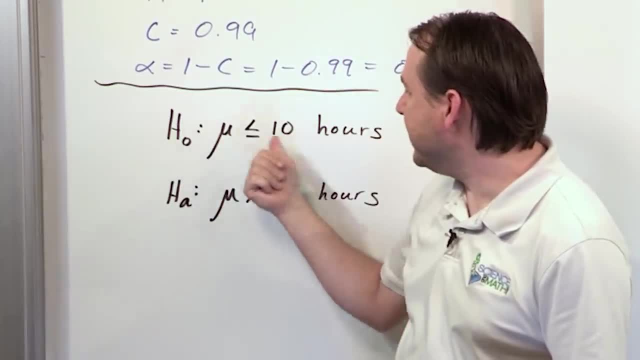 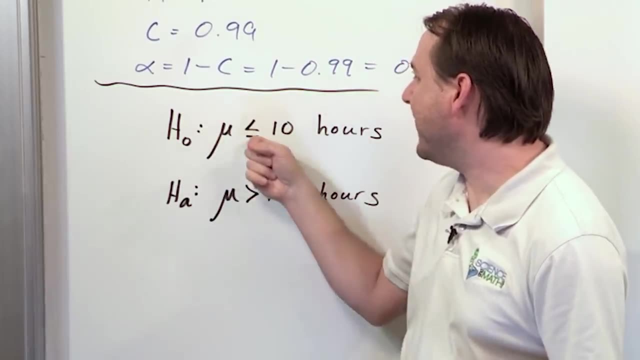 for what could possibly happen. Clearly, a teen, you know, is going to sleep some number of positive number of hours, And so it's either going to be included here, or it's going to be included here And they have to be mathematical opposites. 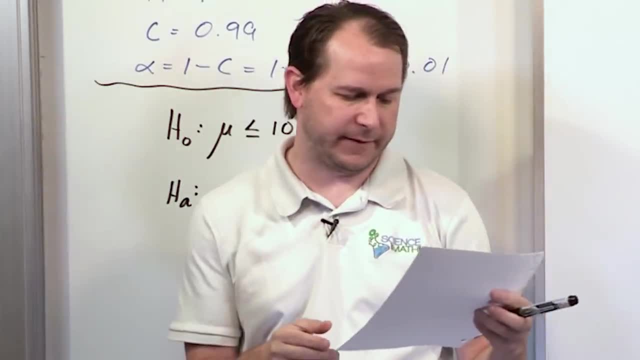 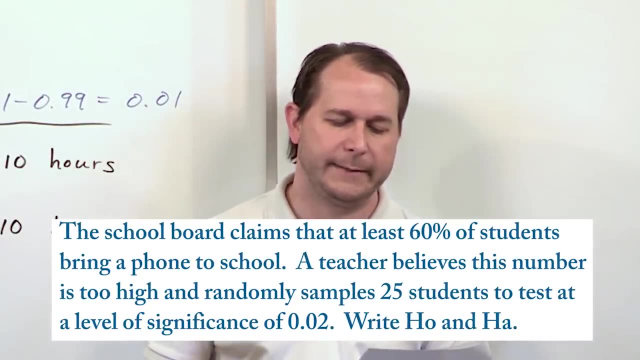 There should be no overlap between them, But together they should encompass everything. All right, Now let's look at another problem. The school board claims that at least 60% of students bring a phone to school. A teacher believes this number is too high. 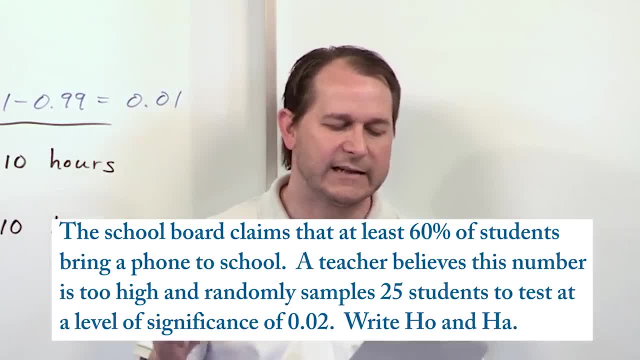 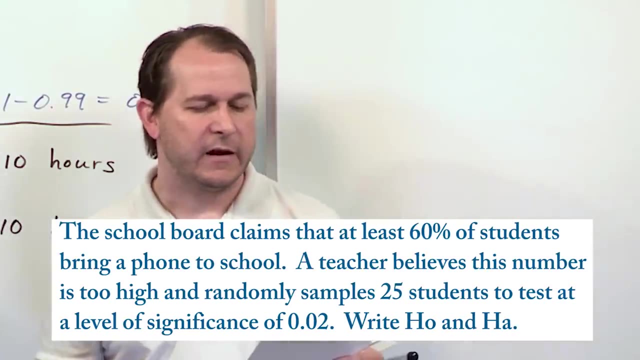 and randomly samples 25 students to test at a level of significance of alpha as 0.02,. what is the null hypothesis H naught the alternate hypothesis H sub A and C, the level of confidence for this hypothesis test. So we're not really asked to perform the test. 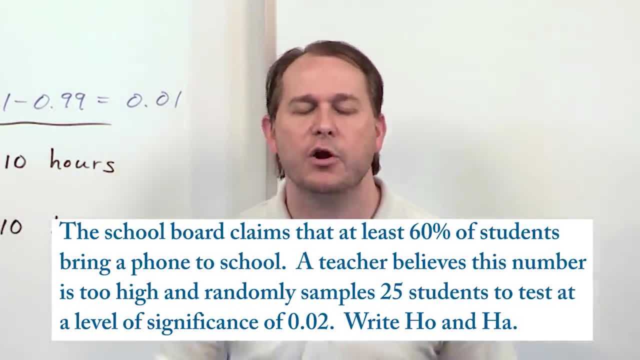 We haven't shown you how to actually test and see if you reject the null hypothesis or not. We just want to set it up and write down the hypothesis. Now notice in this case that what we're dealing with here is percentages. A school board claims that at least 60% of students bring a phone. 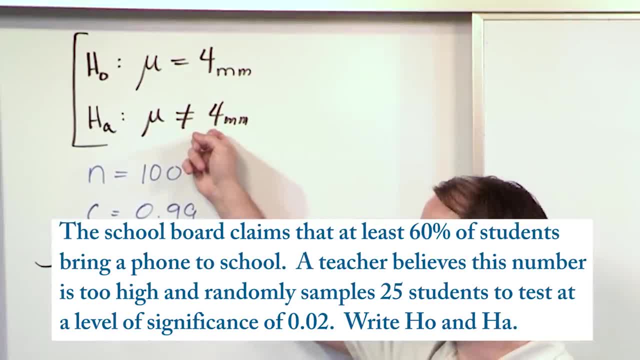 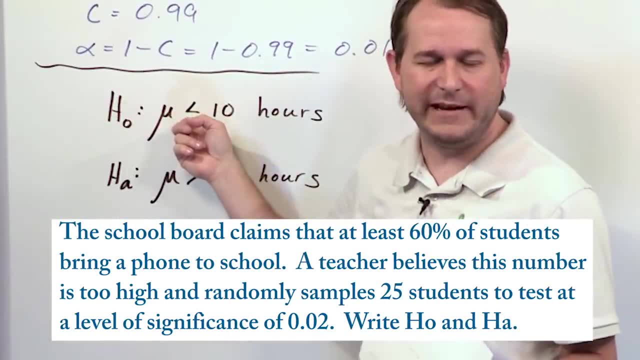 to class. Now, in the previous two problems, this was the diameter of a soda straw, the average value, So that was a number. This was how many hours a student is sleeping, or a teenager is sleeping, So that's a number. So that's why we use mean here mu and mu. 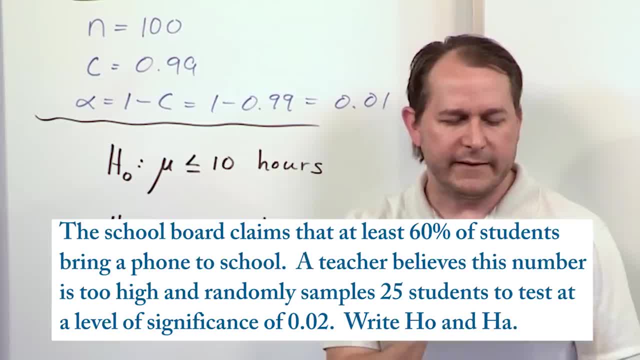 because that's expressing just a number, an average value of something, But in this case it's actually a proportion. Remember, we've done lots of work with proportions. Proportion is just a percentage essentially. You know, 37% of people ride bicycles. 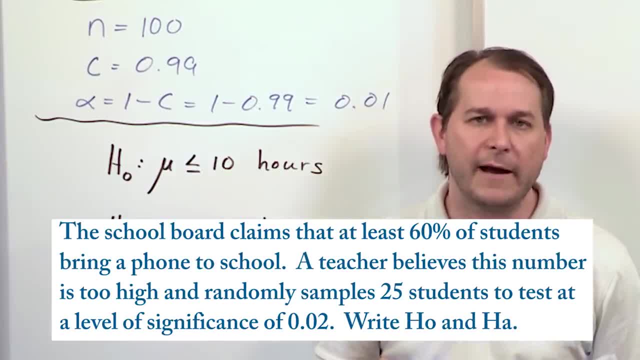 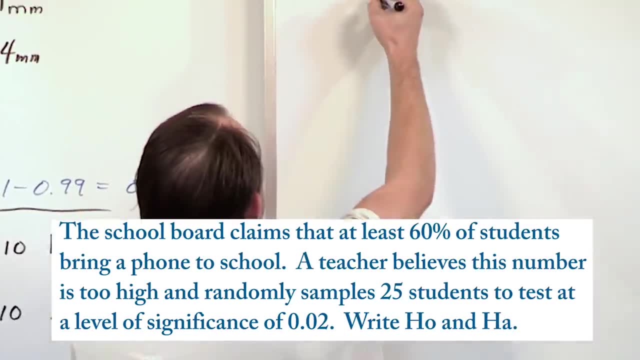 That's a proportion of the population. So here we're going to control the number of students, We're going to construct our hypothesis test, but it's not going to include the mean value of the population parameter. It's going to be concerning the proportion. 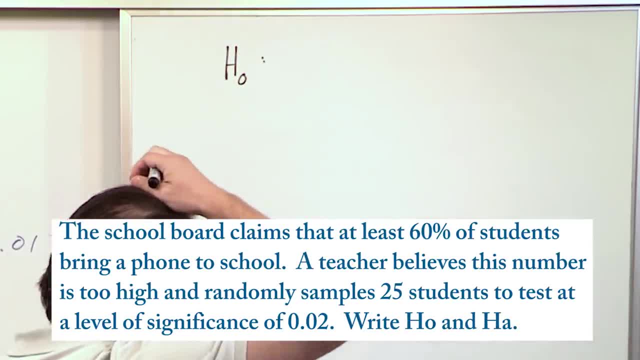 It's exactly the same concept, though The null hypothesis. it says the school board claims that at least 60%- notice the wording at least 60%. So what that means is the proportion of people in that school P is greater than or equal to 60%. 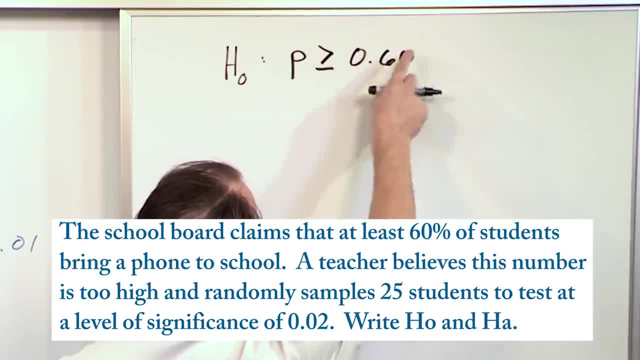 But when we write it down, we want to write it down as a decimal. You don't want to put percent, That's just for our convenience. We want to deal with it in terms of decimals. So you shift the decimal back When we say at least 60%, which is what the wording says. 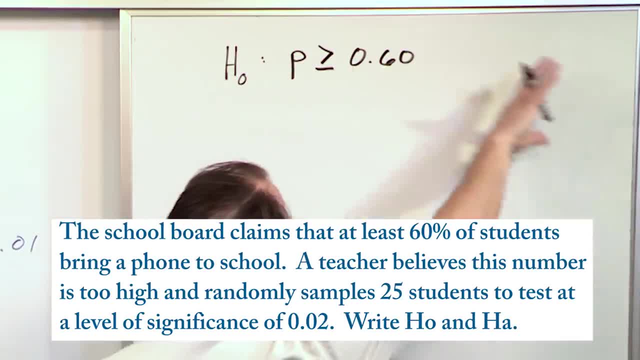 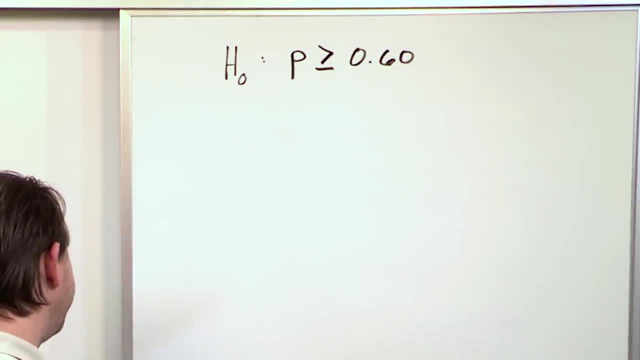 that means greater than or equal to 60%, So anything larger than 60% and also including 60%. that's what the line underneath means. But it says also here that a teacher believes this number's too high. He randomly samples 25 students and blah, blah, blah. 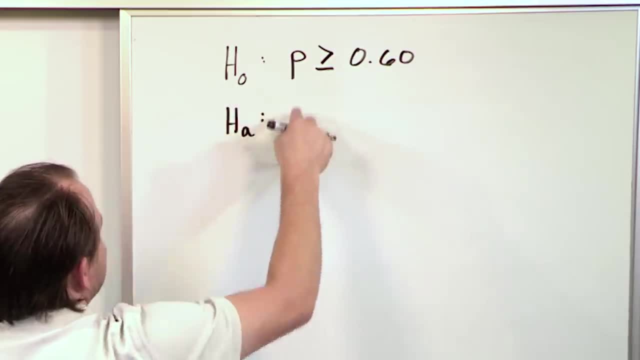 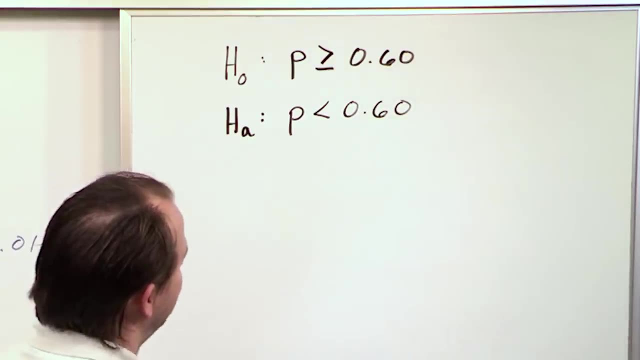 So what would be the alternate hypothesis? Well, they have to be mathematical opposites of one another. so that would mean this one would have to be less than 0.60 or 60%. Notice, there's no equal to here, because that was included here. 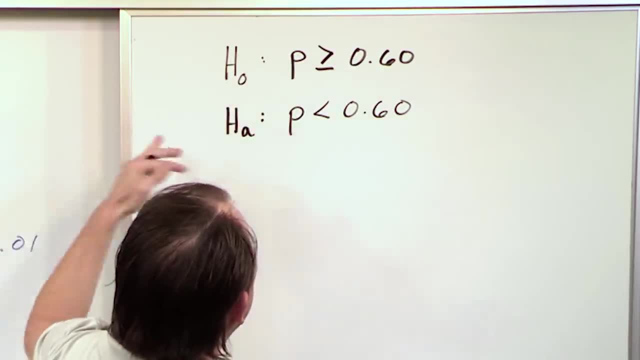 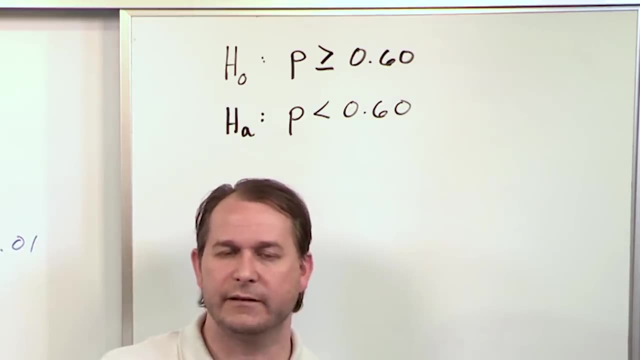 So the top one is the percentage of students who bring a phone is greater than or equal to 60%, And the bottom one is anything less than 60%, but not including, obviously, because that's already taken care of with the first one. 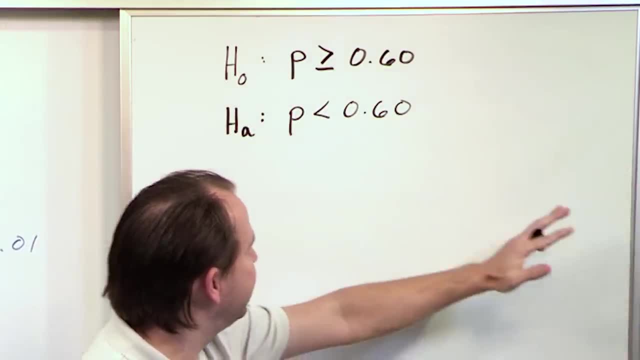 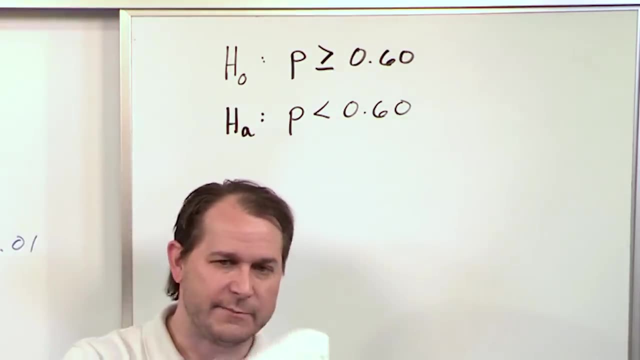 So, again, these are mathematical opposites. This is everything above 60%, and including This is everything below 60%, Not including 60. Together, though, if you kind of line them up like a choo-choo train. 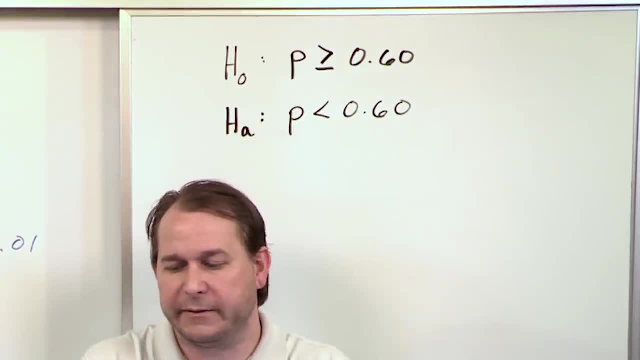 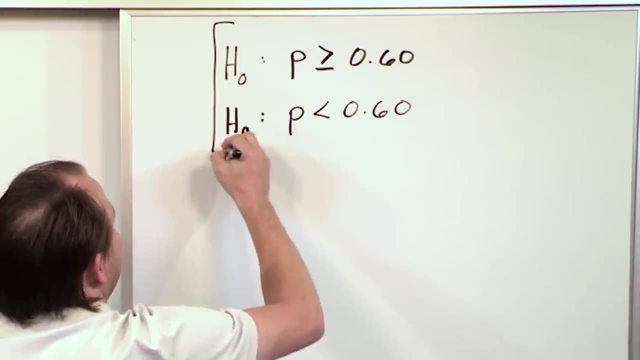 they should encompass all possible percentages that could possibly happen for this problem: the fraction of students that bring a phone to school. So this would be what you would write down for the hypothesis, the alternate and the null hypothesis. This is the status quo. 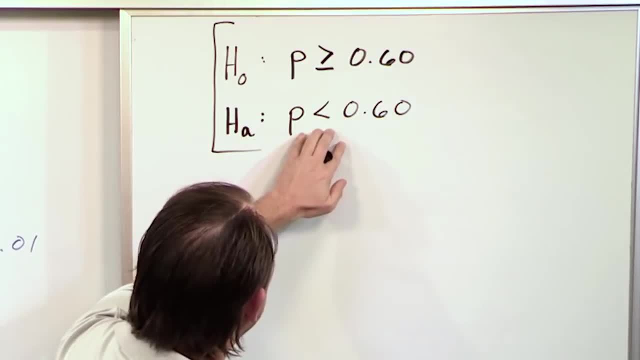 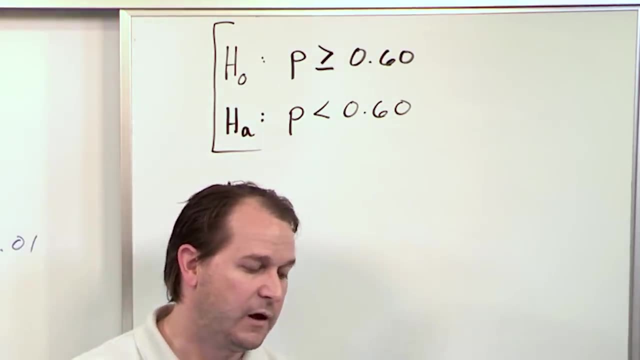 This is what the administration believes to be true. This is a teacher that's researching this. He thinks this is not true. He thinks this number's too high, And so you would set up a hypothesis test. In this case, the problem says: 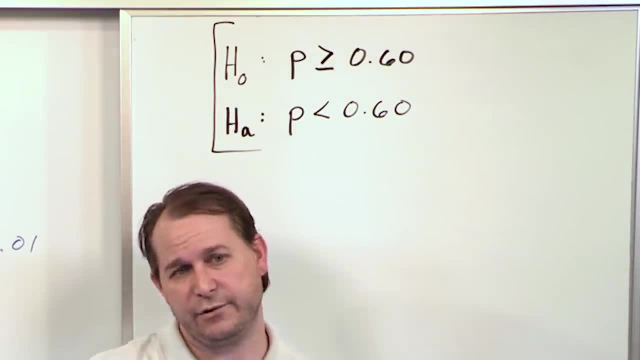 we randomly sample 25 students and we basically just ask them: hey, do you carry a phone to school? We're going to get some data from that. Maybe five people say that they bring a phone to school. Maybe all 25 say that they bring a phone to school. 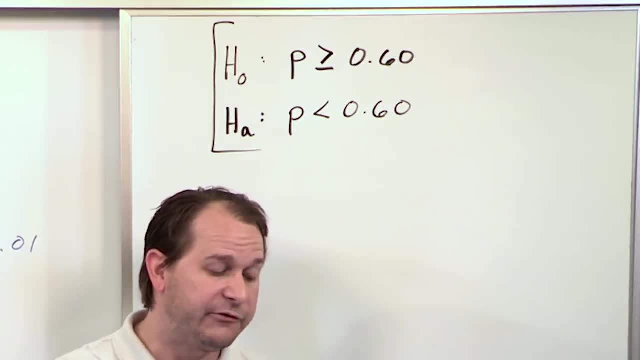 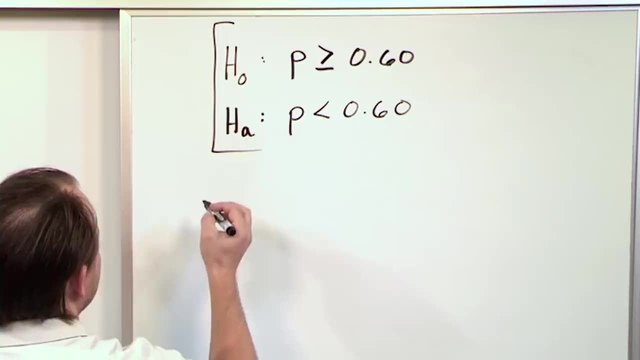 We don't know yet because I haven't given you all of that information, but the teacher does ask 25 students any test at a level of significance of 0.02.. So if when you see something in a problem level of significance, you need to write down alpha and write down exactly what it says: 0.02.. 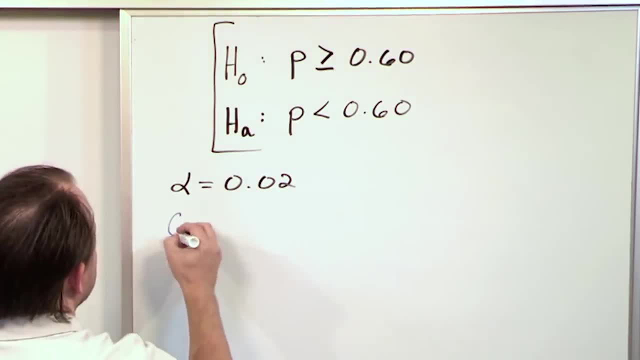 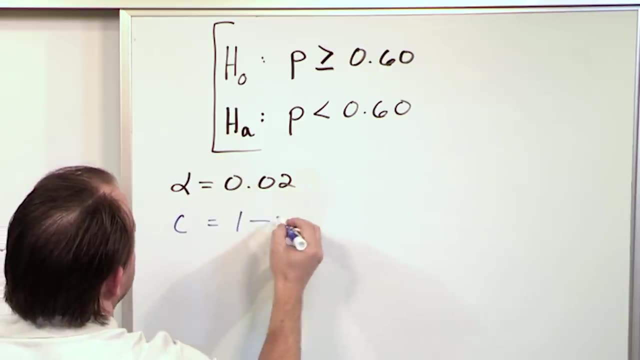 So this problem said: what is the level of confidence? Well, level of confidence, or I should say, yeah, the level of confidence is 1 minus alpha, right, Level of confidence is 1 minus alpha. So basically, what you can do is you can say 1 minus 0.02, so 0.98,, 0.98. 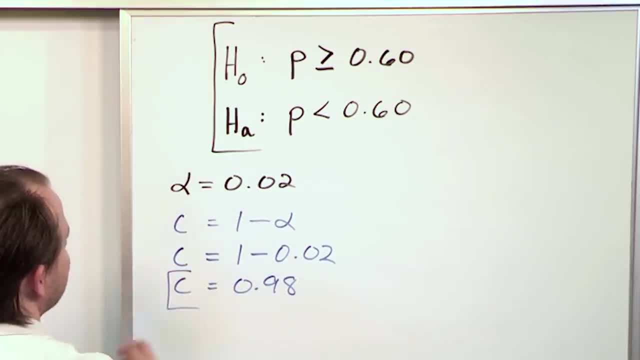 And if you make this in terms of a percentage, it'd be 98%. So this is the level of confidence And you can see again alpha plus the level of confidence. they always have to add to 1.. So that's kind of just something that you always have to keep in mind. 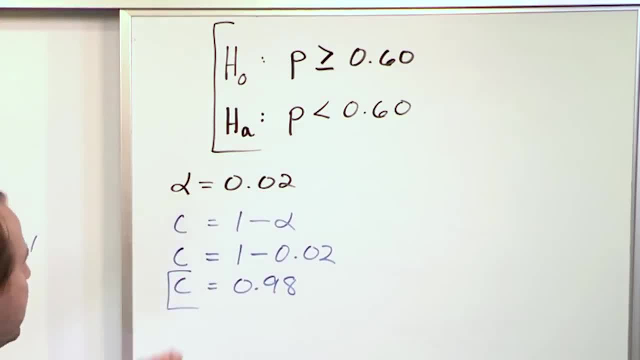 When this is very large, this is going to be very small, and so on. So whether or not the problem gives you alpha or C, it doesn't really matter. You're given basically the same information. You can find the other thing. 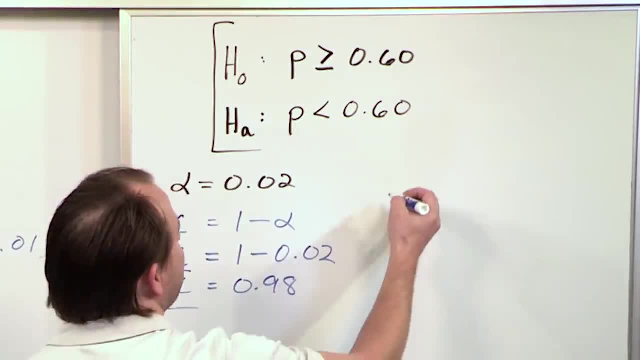 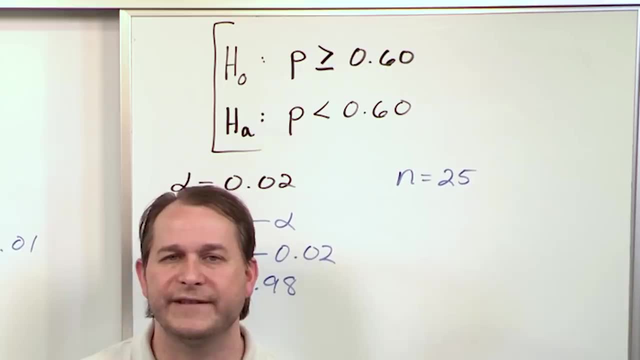 In this case, what is n? The number of samples that you use for your experiment. n in this case is 25.. Now, in this problem, I haven't given you all the information to solve it, because I didn't tell you what the results of your sampling was. 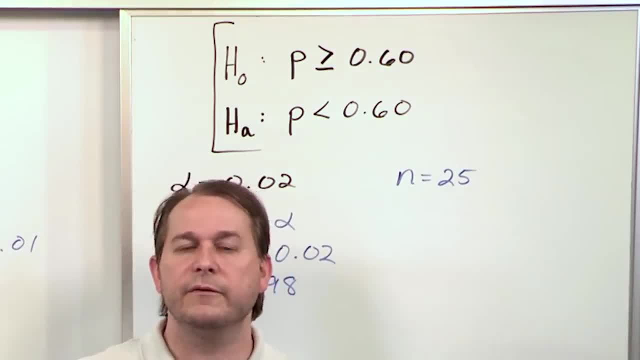 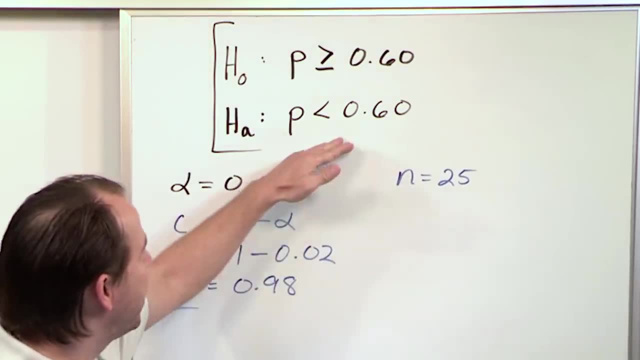 If this were a real problem, I would tell you: hey, you asked 25 students and here's how they answered, And so we have some equation that we'll show you how to use to go figure out how to test this hypothesis using the sample data that you get. 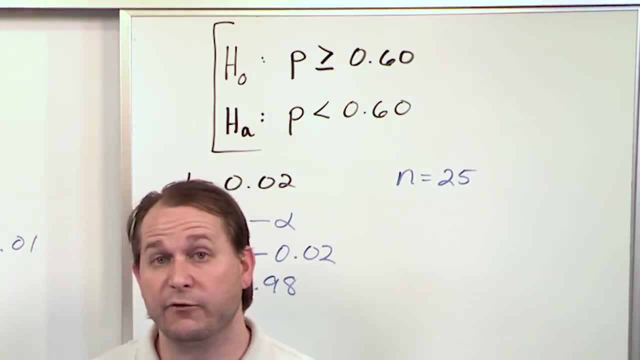 Obviously, you can't ask all the students, but you ask a certain subset of them- 25 in this case. They answer And it's up to you to figure out. when does it become statistically significant? If all 25 of them answer yes, what if 19 of them answer yes? 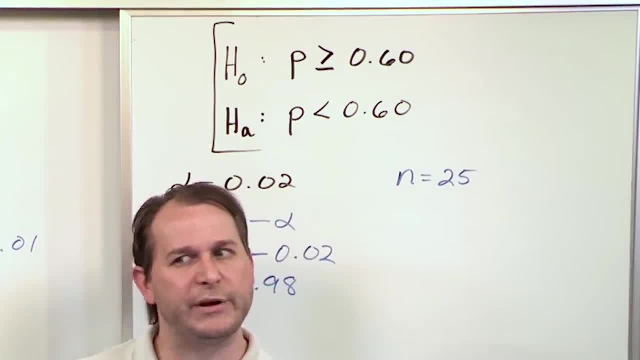 What if 22 of them answer yes? How do we choose the threshold beyond which we're going to reject This null hypothesis or not? How do we choose that? So that's what we're going to get into in the next section. The other thing I'm going to say right before I close is: 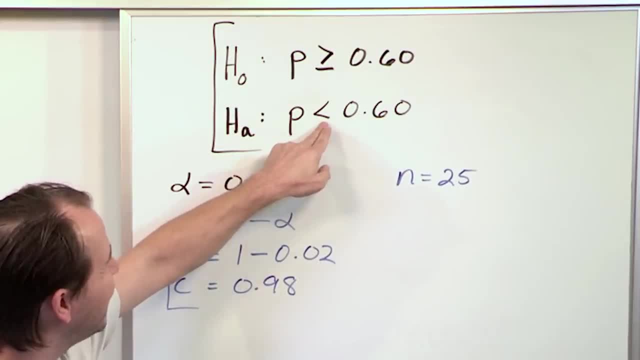 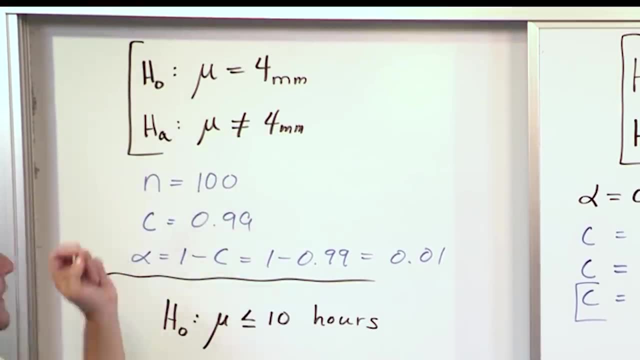 notice that: the alternate hypothesis: sometimes you can get a less than symbol, Sometimes you can get a greater than symbol. in the alternate hypothesis, Sometimes you can get a not equal symbol, Sometimes you can get an equal symbol. So basically, you're going to have equals, not equals. 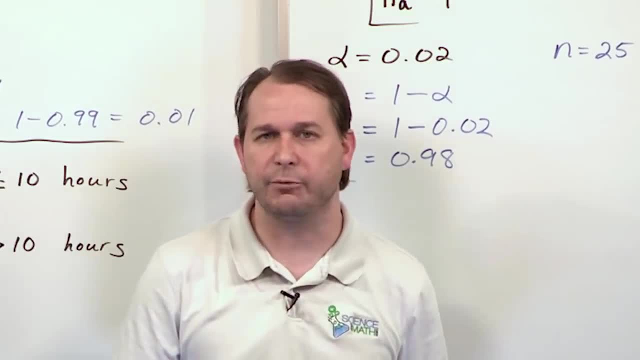 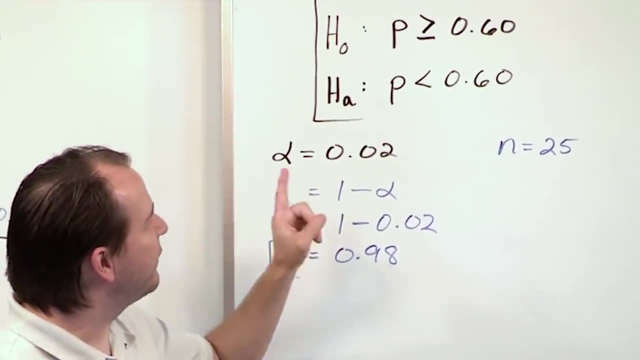 less than or greater than in the alternate hypothesis. That's just the way all these problems are going to fall out, And that's important for you. You need to get right, because what you're going to find out in the next section is the way that you do the hypothesis test. 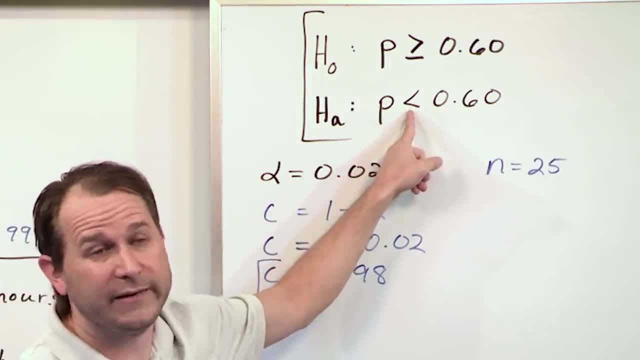 is going to depend on the direction that this arrow basically points. If it points this way, I'm going to show you how to do the test like that. If it points that way, I'm going to show you how to do a test similar. 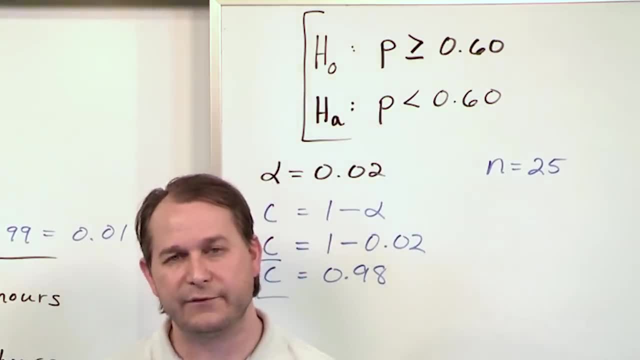 but it's a little bit different And, of course, if it's equal or not equal, you have to know how to handle that too. So the way that you actually do the test depends on this symbol, So try not to get that wrong. 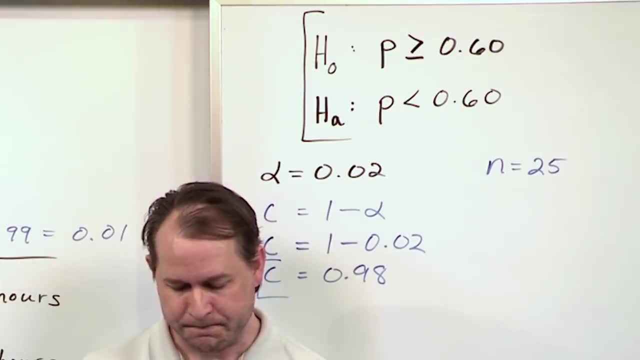 That's why we're doing this practice here: so that you can get confidence with that. This is all I really want to get across to you. We're practicing doing the null and the alternate hypothesis- Very important skill. Follow me on to the next section. 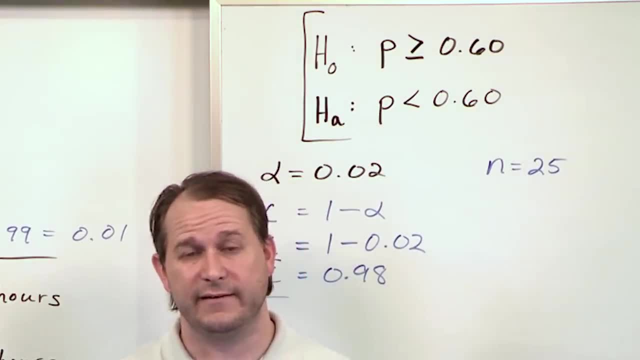 We'll get into a little more of the details on how do you exactly do this testing. Now that you have practiced with what the hypothesis is and how to write them going into the next section, you'll be a lot more comfortable with understanding how do we actually do the testing after we get our sample data. 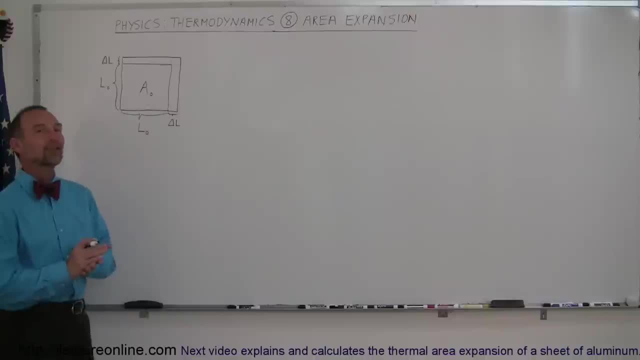 Welcome to Electron Online. Next we're going to look at area expansion. Of course, expansion due to thermal expansion. Thermal increase of heat causes atoms and molecules to vibrate more. Everything expands. So now we're going to look at the expansion in an area rather than just a length. So let's say that this was our original area. We heat up that plate. Let's say it's a plate, a thin plate. Then it's going to expand in all directions. Of course we're only going to look at the expansion in one direction. here Makes it easier to do the mathematics, And so let's say that each length increases in one direction. 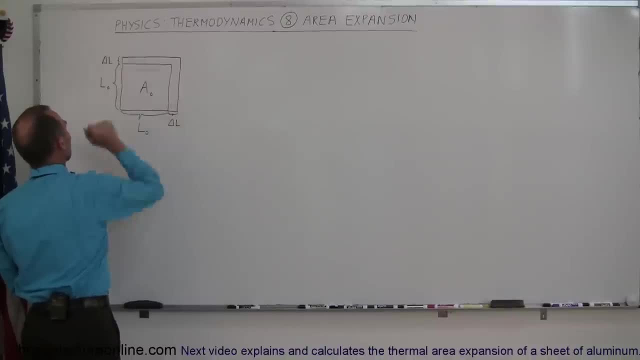 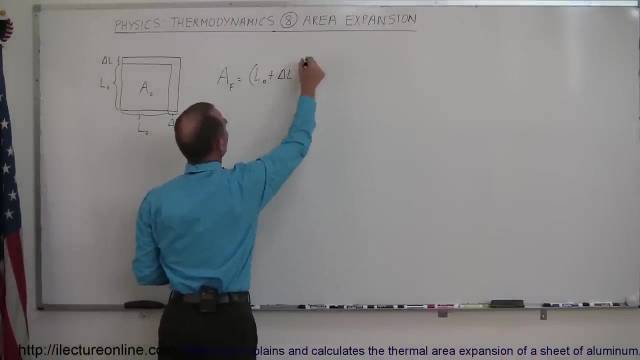 Increases by a small amount of delta L in this direction and delta L in that direction. So the new length or the new area- I should say A final- is going to be equal to the product of the two sides, of course. So it's going to be equal to L sub naught plus delta L, quantity squared. If we now go ahead and square that quantity, it's binomial. So this is the first term squared plus twice the product of the two: Two L sub naught, delta L times the last term squared. 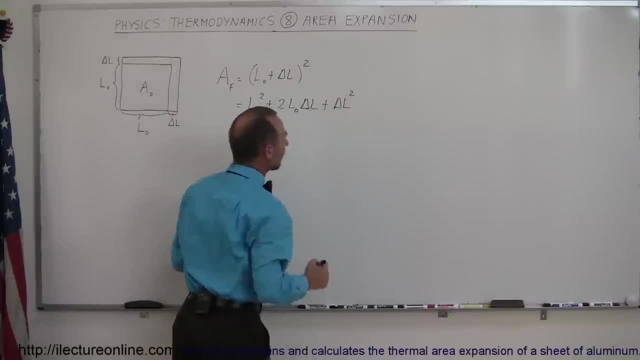 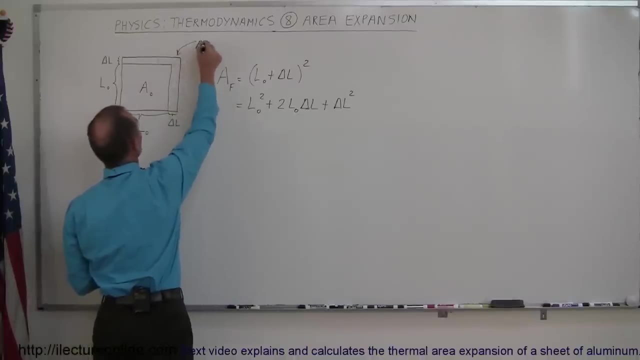 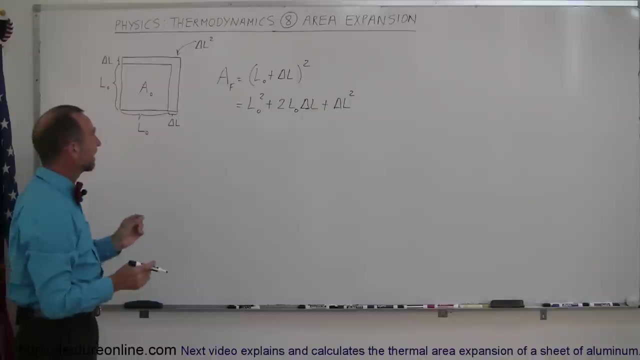 So plus delta L squared, Now delta L squared is going to be a very small quantity. That's this little thing right here at the very edge. So this is a delta L squared. Notice the L sub naught times delta L, Those are the two long stretches right here And of course your A sub naught is simply your L sub naught, squared right there. Now turns out that the delta L is so small we can probably just ignore it, So we're just going to assume that this is approximately. 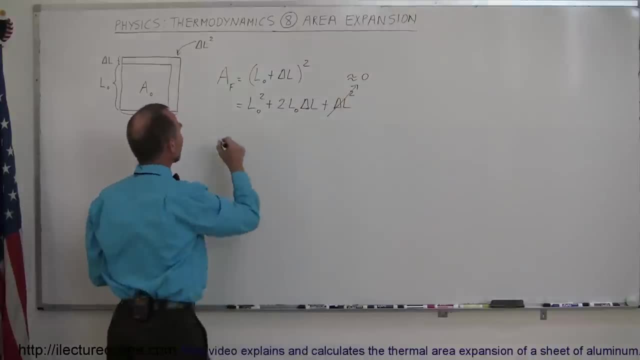 equal to zero, And so we can just ignore it, Which means that the final area is simply going to be equal to L sub naught squared, plus two L sub naught delta L. Now, this L sub naught squared, of course, that's the original area, So we can say that A final is equal to the original area plus two L sub naught delta L. Now, next, what we need to do is look at this delta L right here. So what is delta L?